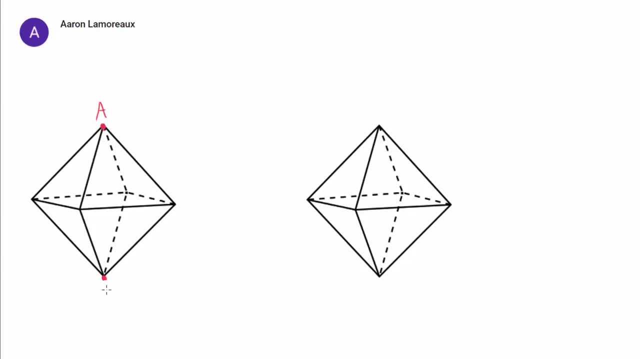 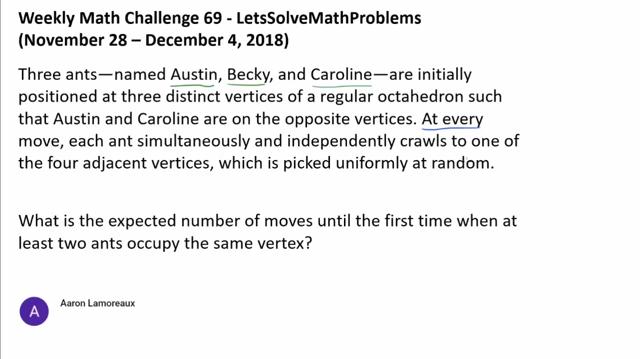 of generality, Let's say Austin is at the top, then Caroline is at the bottom And we are not specifying where Becky is. so, for example, this is one place she can be at. At every move, each ant simultaneously and independently crawls to one of the four adjacent. 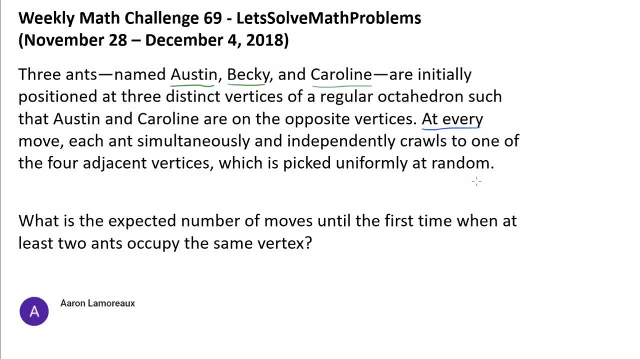 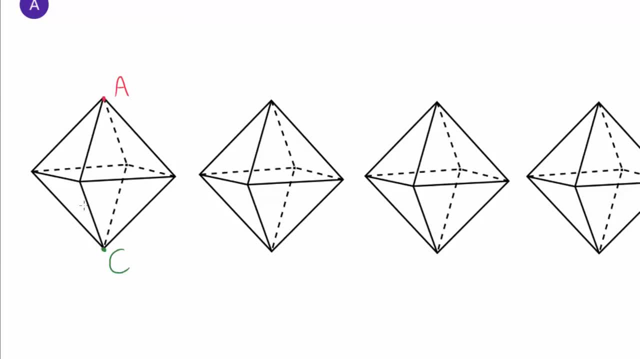 vertices, which is picked uniformly at random. So if we take a look at this diagram, we know at the beginning Austin and Caroline are opposite each other, while Becky is at one of the middle vertices. without loss of generality, This is one possible verse. 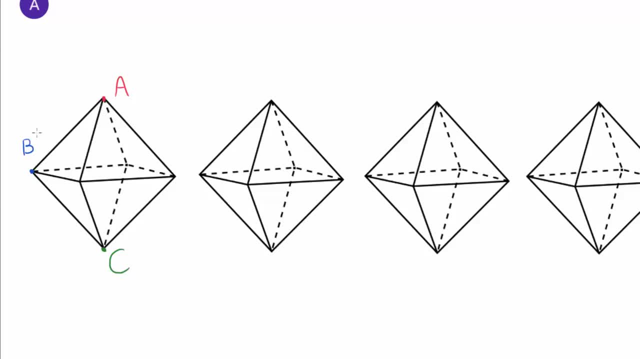 position a, b, c can occupy, and after that, after this initial position, the ants are going to start moving around this octahedron following some edges. so here's one possible example of how this can play out. so in this particular example, a is moving down this edge to here, b is moving to this. 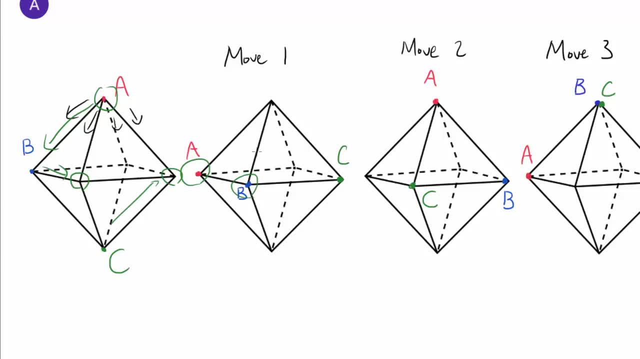 one, while c is going up to this one. so after move on, this is the configuration and they can move one more time. a is going back up, b and c are trading spots in this case, and after one more move we see that b and c occupy the same spot, while a has moved back down. let me scroll to the right just. 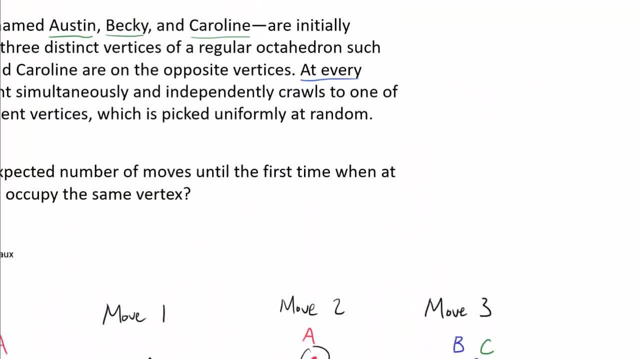 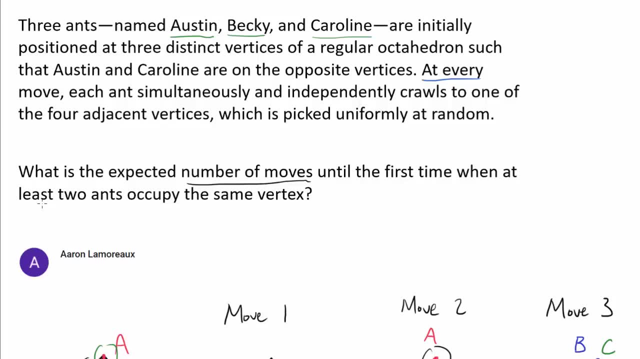 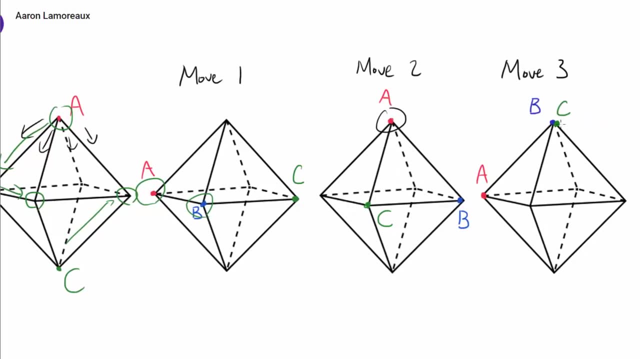 in case you cannot see, so now, let's go back up. so we wish to find the expected number of moves until the first time when at least two ants occupy the same vortex. so in our example we know the number of moves it took until until at least 2 ants occupy the same vertex is 3.. 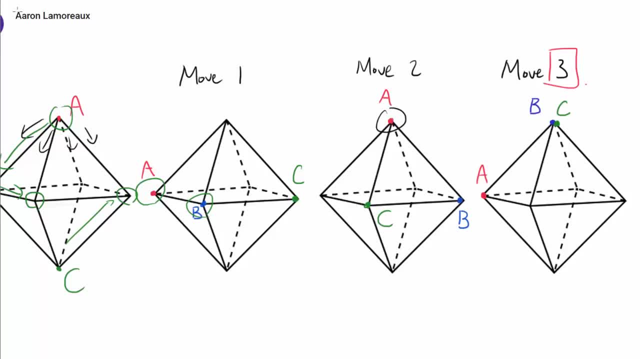 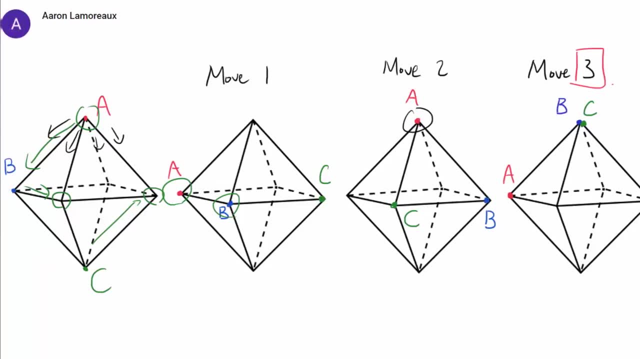 But that's not what we want to find. we want to find the expected value or the average number of moves. it's going to take until at least 2 of them are on the same vertex Before we proceed to the solution. I want to take this time to recognize Aaron Lemura. 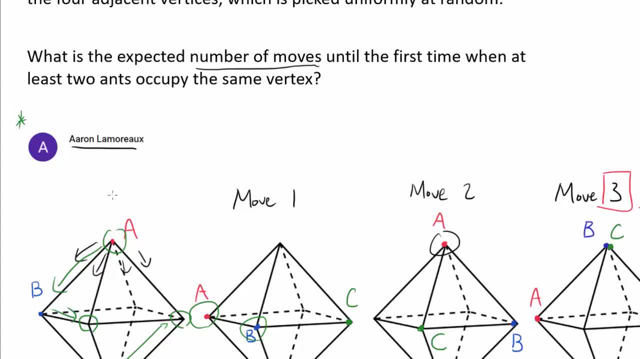 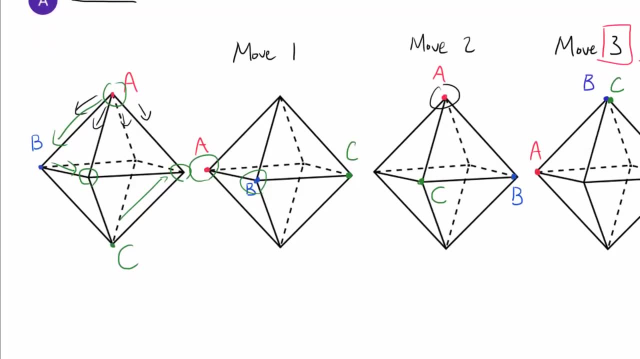 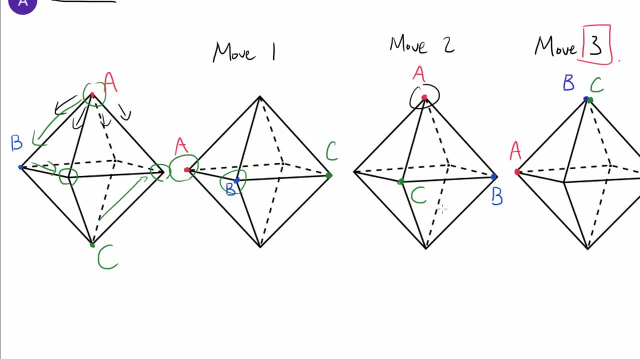 who was the very first person to post the correct answer to this challenge problem. A huge congratulations to Aaron. So now let's go back to this problem and let's think about how we can approach it, Examining this diagram and thinking about the situation with 3 ants on an octahedron. 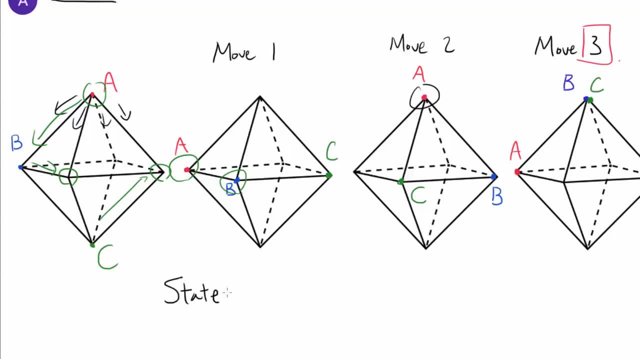 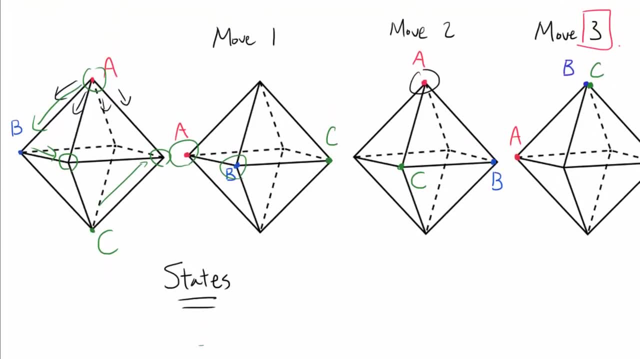 we see there are only 2 possible states of how ants can be configured on the octahedron. And what do I mean by this? I assert that before the ants are together. so starting at the initial position and disregarding the final position where we stop. I assert that either 1., 2., 3., 4., 5., 6., 7., 8., 9., 10., 11., 12., 13., 14., 15. 16.. 17., 18., 19., 20., 21., 22., 23., 24., 25., 26., 27., 28., 29., 30., 31., 32., 33.. 34., 35., 36., 37., 38., 38., 39., 39., 40., 41., 42., 43., 44., 44., 44., 45., 46.. 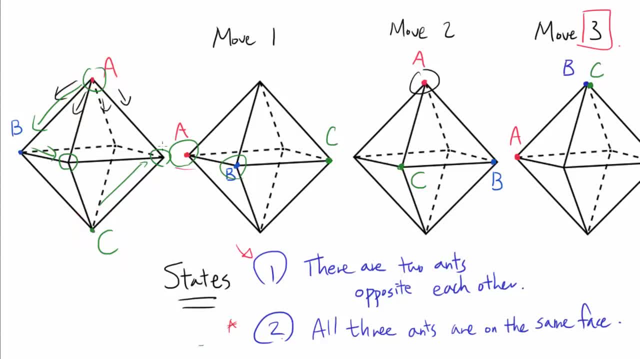 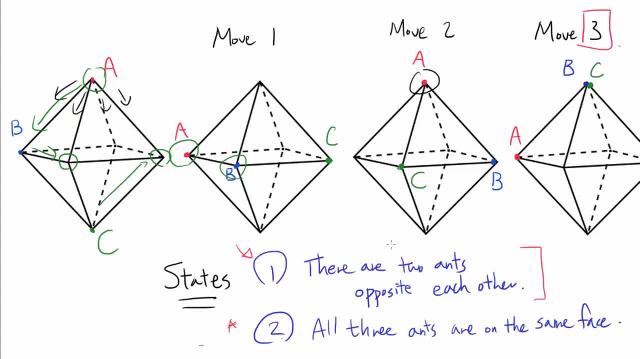 100. 100. 100. 100.. Think about this for a moment. but it's not too hard to see that if we cannot find the two ends opposite each other, then every single end should be on the same face. So in this case, we have state two. 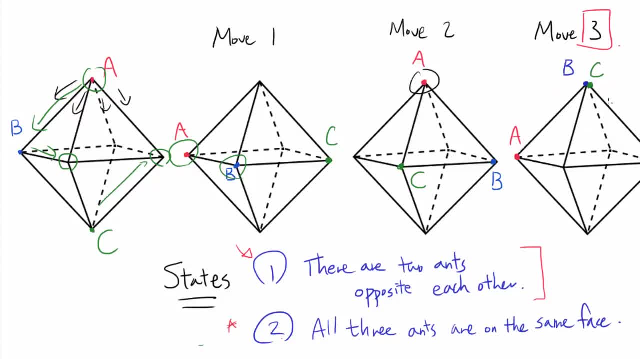 And at the end, of course, at least the two ends are together. So, basically, what's happening is that we are starting at state one And we are going to have a sequence of state one and state two- In this case, state 1,, state 1, state 2, until we get the configuration that we want. 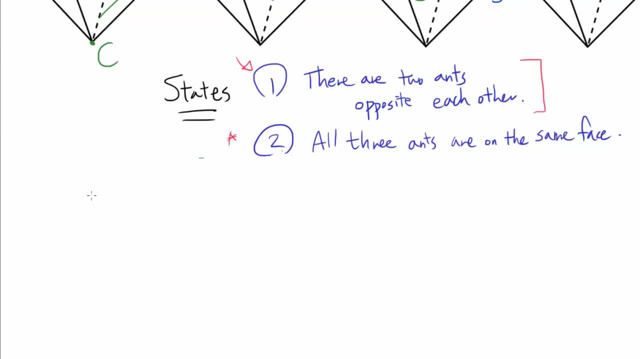 So here's how we can break this problem down. Let's say mu1 is the expected number of moves from state 1 until we get to the end, And let's say mu2 is the same thing, except that we are in this case looking at state 2.. 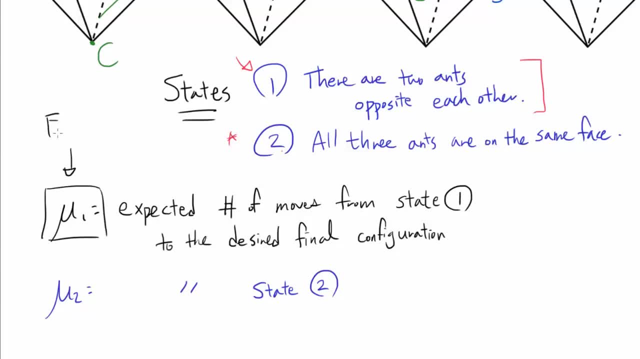 So we want to find mu1.. So this is what we wish to find: Once we find mu1, we are done. And it turns out, introducing this mu2 is going to help us find mu1 as well. So how? so? Well, think of it like this: 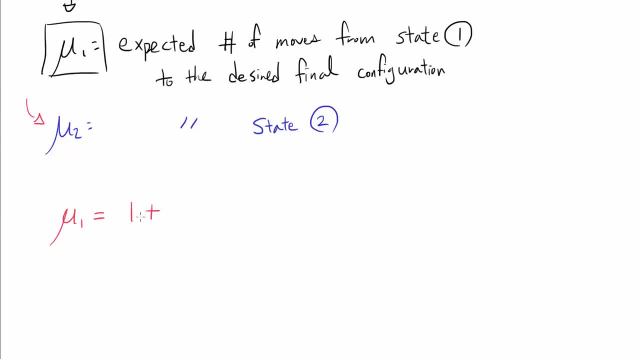 Starting in state 1, we are going to start by making one move And with some probability. we don't know what the probability is, So this is some probability that we are going to fill in later on, Some probability that we are going to stay in the state 1.. 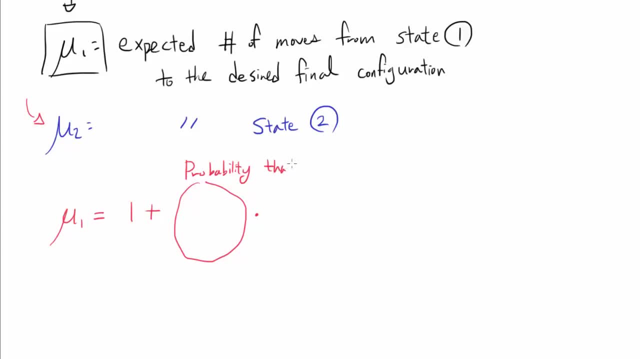 So this is the probability that We are going from state 1 to state 1.. And once we go back to state 1, there is mu1, more expected values to go, Or there is some probability. I'm writing this giant circle. 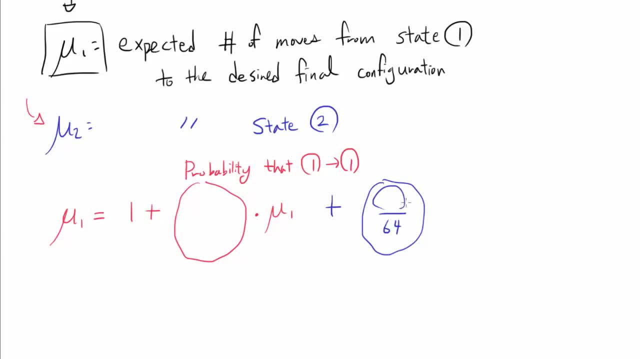 but that's where the probability. some number is going to go in later on, Who knows, like 20 over 64.. So this is the probability that we are going from 1 to 2.. So state 1 to state 2.. 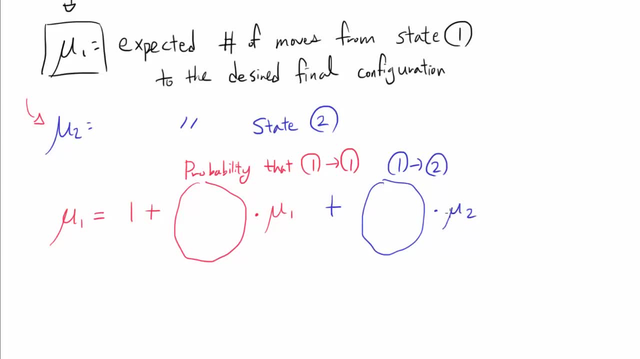 And then we are going to have to go mu2.. And then we are going to have to do two more steps on average until the end. So we know mu1 is equal to this thing. So once we can find the probability that we go from state 1 to state 1, and state 1 to state 2,, 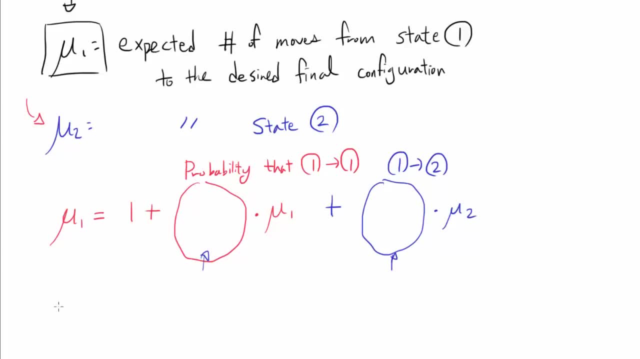 we have this equation relating mu1 and mu2.. And we can do the same thing for mu2.. mu2 is going to be 1, plus some probability that we are going to go from state 2 to state 1, times mu1,. 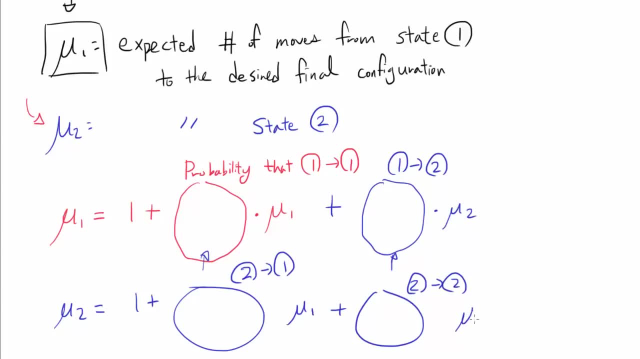 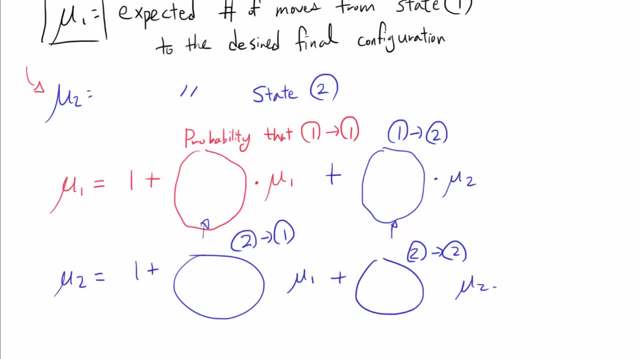 plus some probability that we are going to stay in state 2, times mu2.. And then, Once we find the probabilities, we are going to have this system of equations- system of linear equations, in fact, in mu1 and mu2, which we know how to solve. 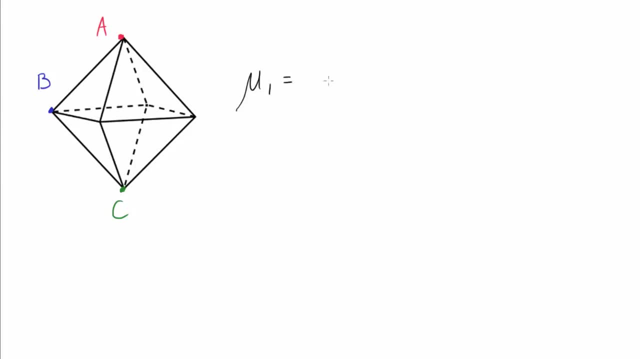 So let's find the probabilities. So we are going to start with mu1.. So that's 1 plus 64 over something that we are about to find, times mu1, plus something over 64 times mu2.. It's over 64, because A has four choices. 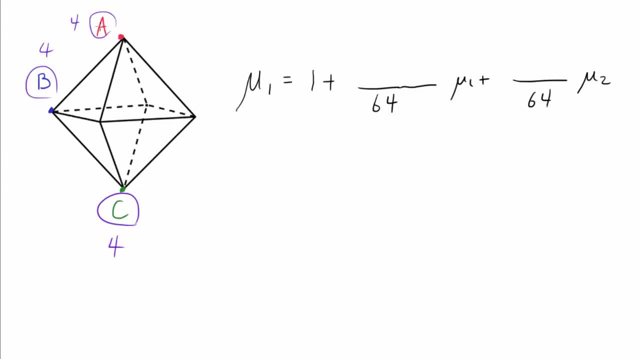 B has four choices And C has four choices. choices 4 cubed 64. so we are going to be dividing by 64. now on the numerator, we want to find the number of ways we can go from state 1 to state 1. now to count this, i'll do some case work, let's. 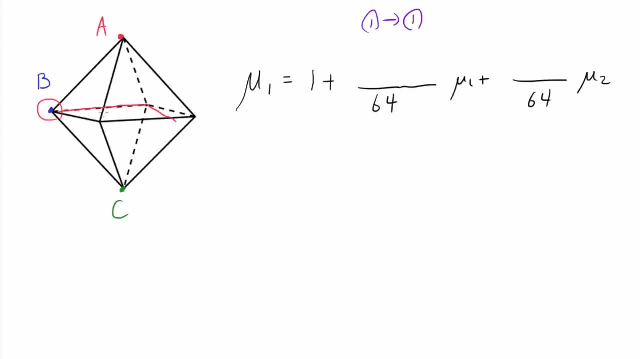 first count the case where b is going to stay in this plane, in this square, and as a sub case, number 1, let's consider the case where b and a or b and c are opposite each other after the move. so we know b has two choices of where to go and we have two choices on whether to pick a or c to be opposite. 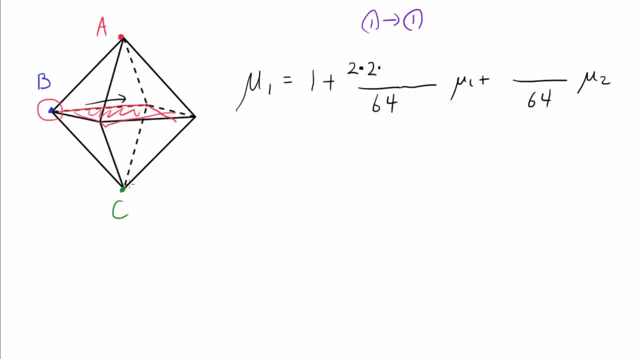 of b, and once b moves we know, whether a or c is picked, that that chosen a or chosen c has only one choice: to go opposite b. so times one and the other one. so if a is picked, a has to go opposite b. that's one choice, but the other one still has two choices. so two times two times two. now let's. 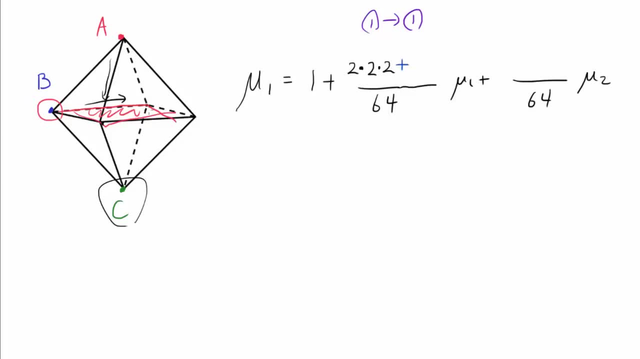 consider the case where b is still still staying on the same horizontal plane, but this time a and c are going to be opposite each other. so in this case b has two choices on where to go and after b moves, for example, here we have exactly one pair of points where a and c can go, but we can either have a, c or c a, so that's two. 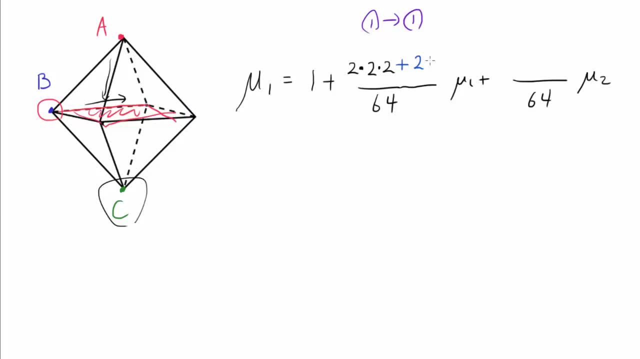 more choices, so we want to multiply that by two. and finally, let's consider the case where b is going to go up or down. so we have two choices on whether b is going up or b is going down, and after b moves, obviously a and c cannot occupy this vertex at. 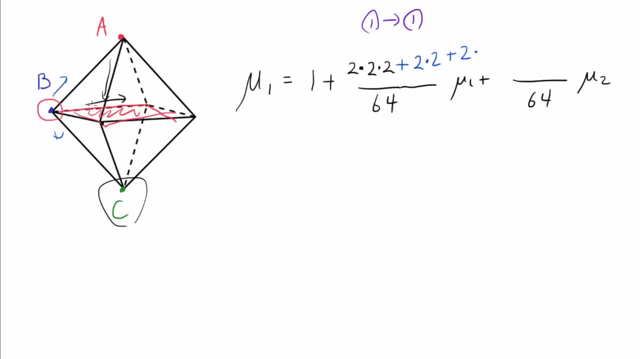 the bottom. so a and c have to be opposite each other. so there are two different ways we can choose the opposites, like this or like this. so that's two different choices, and within the two choices we have two more choices on where to put a and where to put c, and we see that this entire 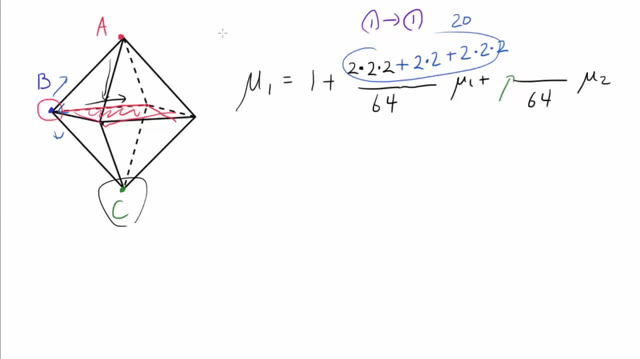 thing adds up to 20. now let's look at the second fraction, where we want to count the case where we are going to be putting a and c together. so let's look at the second fraction, where we are going to going from state 1 to state 2 and we can count this the same way. let's start by considering the. 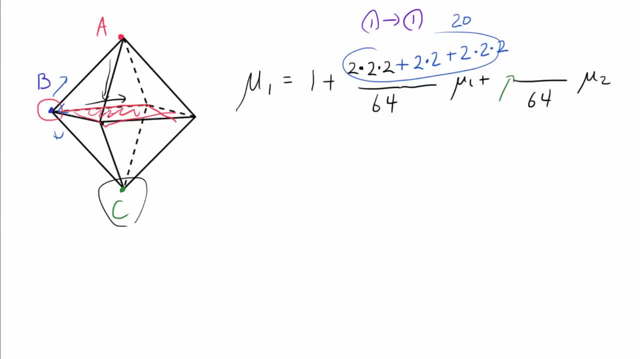 case where b is going to stay in this same horizontal plane, but realize if b is staying on the same plane, well, a and c are going to join b on the same plane. and because we have four points here and we have a, b and c coming down on this plane, at least two of the points have to be. 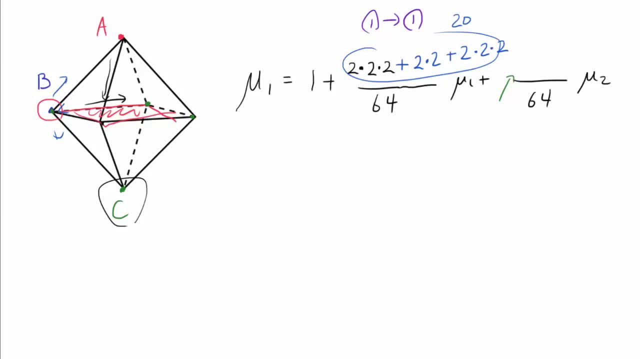 opposite each other, which we do not want. and this is implying that b has to go up or go down. so we have two choices for whether b goes up or b goes down. and after b moves, the only restrictions on a and c are that they have to be adjacent to each other. so, like this, like this, like this or. 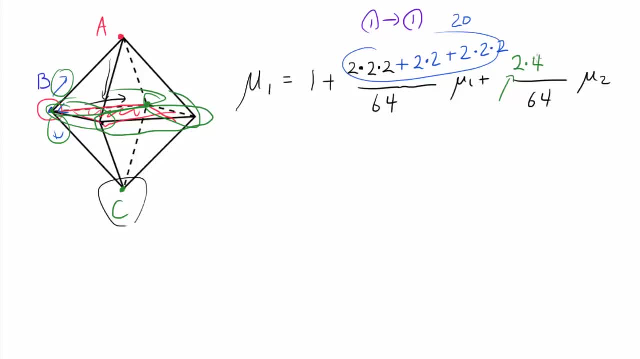 like this. so there are four different choices and in each of those cases we have two different ways of ordering b and c, b, c or c b. so we have two times four times two or 16, two times four times two or 16. so in this case we have two different ways of ordering b and c b, c or c b. 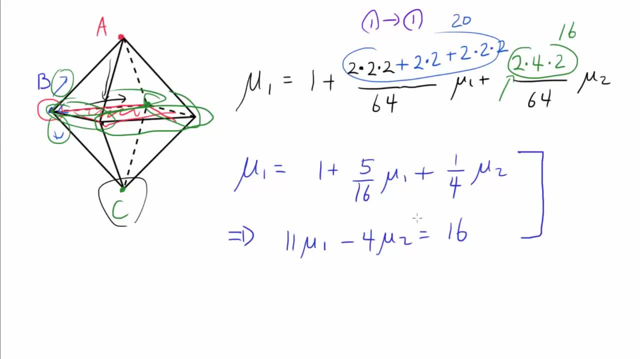 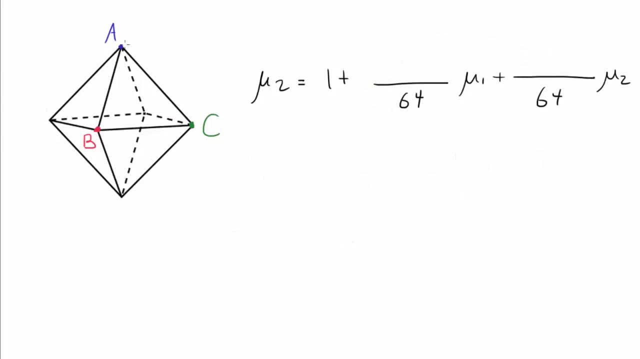 ways. in this case I did a little bit of simplification off camera and this equation is equivalent to this equation: 11 mu 1 minus 4 mu 2 is 16.. We are halfway done. Now let's consider the case where we start with state 2, where a, b and c occupy the same phase. So in this case, to go, 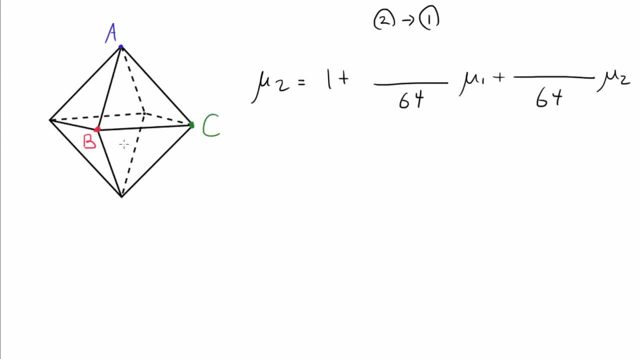 from state 2 to state 1. what do we have to do? Well, let's use casework one more time. Let's first consider the case where both b and c are going to stay on this same horizontal plane, So both b and c are going to move left or right. It's not too hard to see that b and c cannot be opposite each. 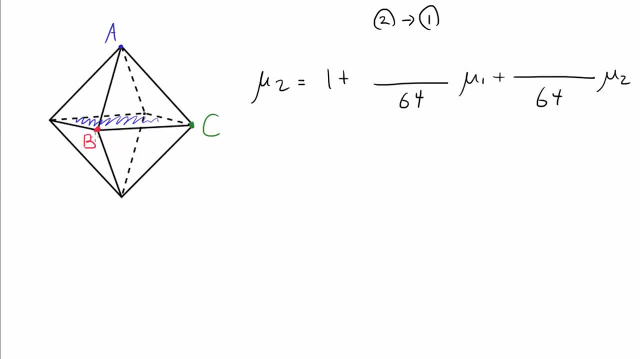 other after the move. So it's either going to be a opposite b or a opposite c. So we have two choices, either b or c to be opposite a. So, for example, if it's b, we have two choices for where b can go and we have only one choice for a. 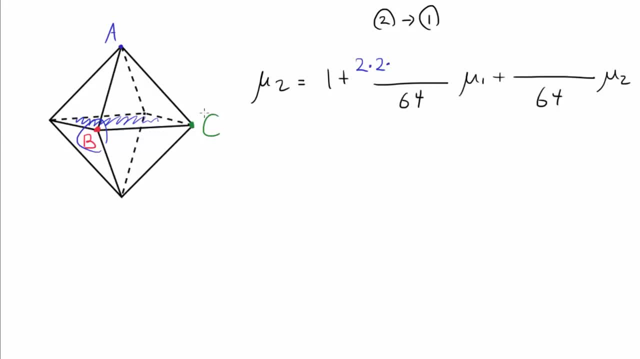 go opposite b or opposite c, depending on which- and it's not too hard to see that movement of b and a opposite b is not going to interfere with c. it's not going to place any restrictions on where c can go. so we still have two choices for c. now let's consider the case where one, b or c, is going. 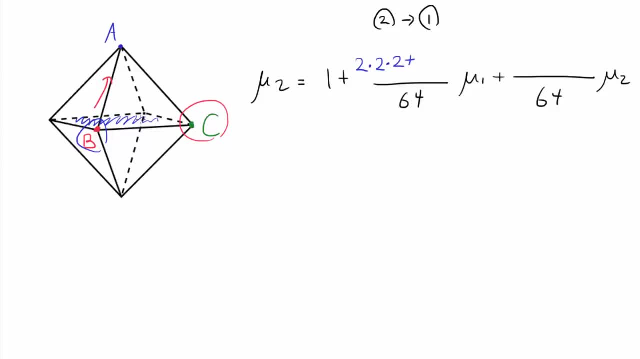 to move up or down, while the other one is going to remain in the horizontal plane. so in this case we have two choices on whether to pick b or c to leave the plane, and that chosen point either can go up or down, and c can move anywhere in the plane and a is going to come down opposite c. 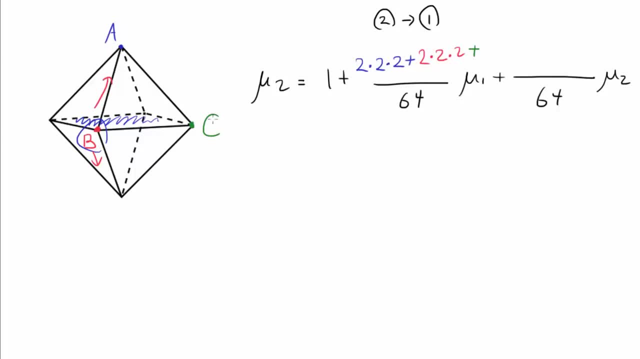 so we have two times two times two. and finally, the last possibility is where b and c are going to both leave the plane. so either b is going to go up and c is going to go down, or vice versa. so we have two choices: whether b goes up or c goes up, and once b and c moves, they are opposite each other. so we have a four choices. 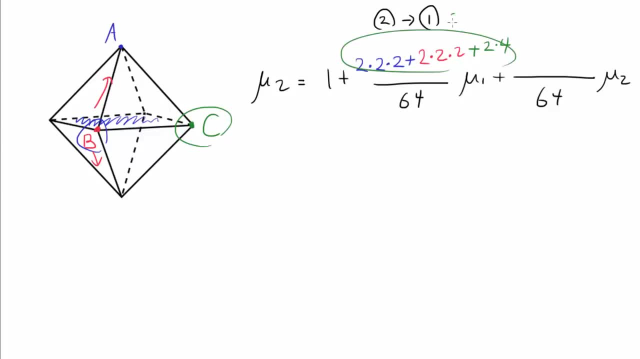 for a. so here, if you add it up, we get a total of 24.. we are so close. let's take a look at the final case where we want to go from state 2 to state 2. so by the end of this move, we want a, b and c to be. 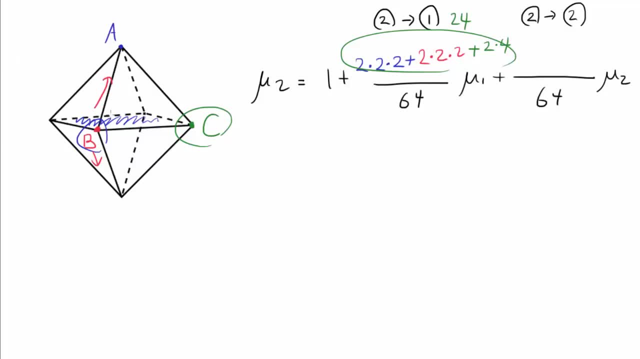 adjacent to each other one more time, and here, once again, both b and c remaining in this horizontal plane is out of the question. so let's take a look at the final case where we want to go from state 2, because in this case, a is going to join them in the plane and we are going to be able to find two. 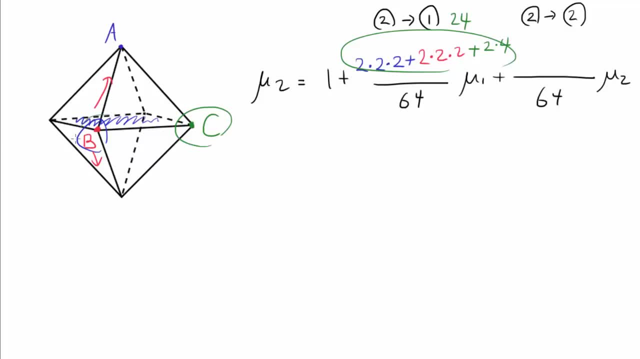 of them that are opposite each other, and we can have both b and c leaving the plane, because then they are going to be opposite each other. so exactly one- b or c- can move up or down. so we have two choices, b or c, and we have two choices for up or down, and after that the other point has: 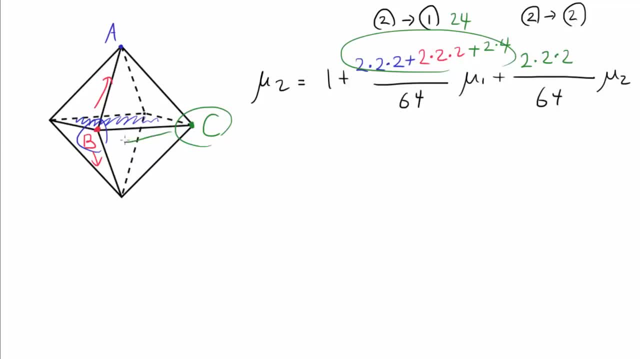 two choices on where to go in the plane, and no matter where that point goes, it has two choices, one to the left and one to the right- to come down adjacent to the point. so we have, in this case, 16 possibilities. and now let's simplify this equation. this is what i got: 6 mu 1. 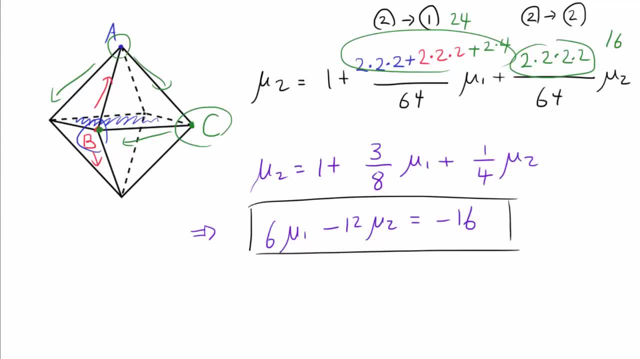 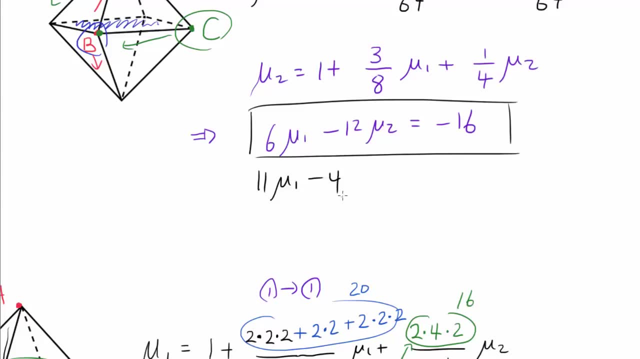 minus 12 mu 2 is negative 16. i can actually divide this by 2, but this is good enough because we have the other equation being 11 mu 1, 11 mu 1 minus 4 mu 2 being 16. yes, it is, and realize that we wanted. 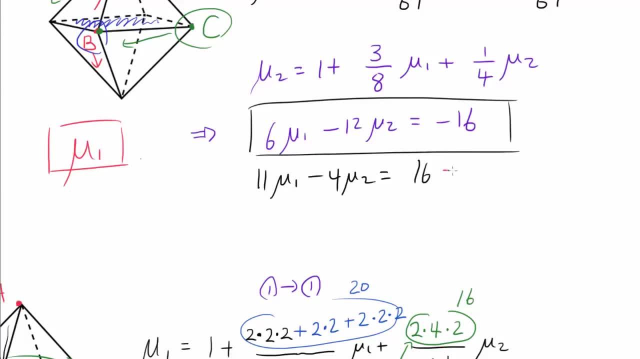 mu 1. once we find mu 1, we are done. and that's easy to do. multiply this equation by 3: 33 mu 1 minus 12 mu 2 is 48. do this equation minus this equation, getting us: 27 mu 1 is a 48 plus 16 or 64.